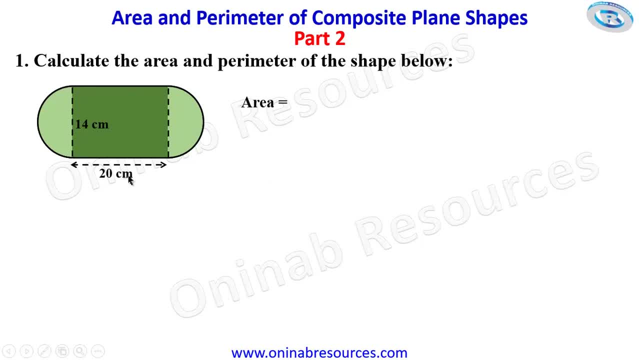 Area of a rectangle is length times breadth. That's going to give us 20 times 14.. Taking care of the area of the rectangle, then we now look at the area of the two semicircles. The two semicircles, when joined together, form a circle. So we then find the area of 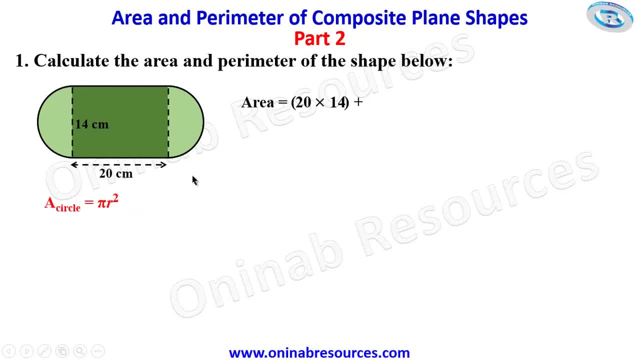 a circle. Area of a circle is Pi R squared, and our R is 14 divided by 2, because radius is diameter divided by 2.. So we are going to have the area of the two semicircles as 22 over 7 times 7 over 1. times 7 over 1. 7 goes with 7 to give us 1. 7 goes with 7 to give 1.. So we are left with 1, 7 goes with 7 to give 1, 7 goes. 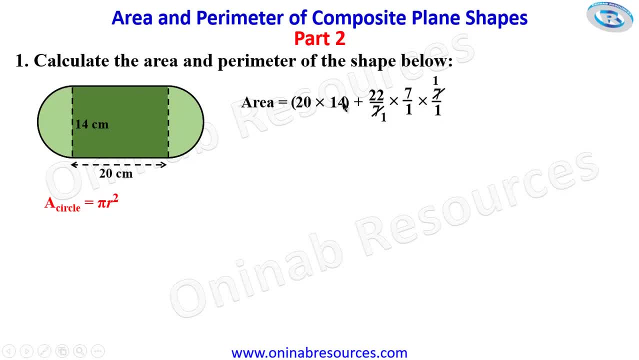 1.. 7 goes with 7 to give 1.. 7 goes with 7 to give 1.. So we are left with 2, 7 goes with 1.. We already have 1.. Therefore���, Al De souci about this area and the surgery with the contract. The problem is that this surface aspect and this pressure isACH is too low. 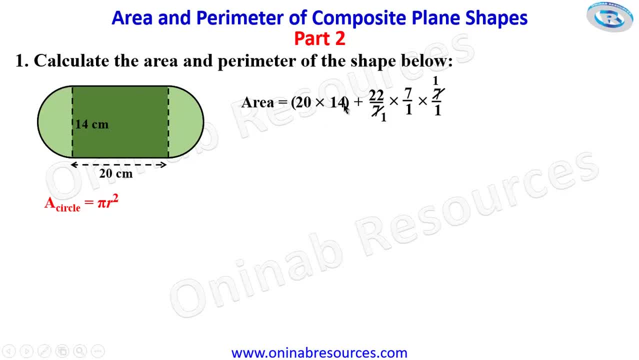 22 times 7 here and 20 times 14.. 20 times 14 will give us 280, then plus 154, since 22 times 7 gives 154.. We are adding the two areas, since the shape is an attachment of two semicircles to a rectangle. 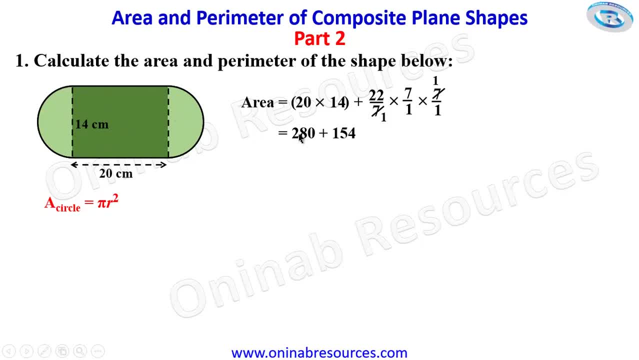 on both sides of the breadth, Adding 280 and 154, we have 434 square centimeters as the area of the shape. So we have the area of the shape to be 434 square centimeters. We then go ahead to find the. 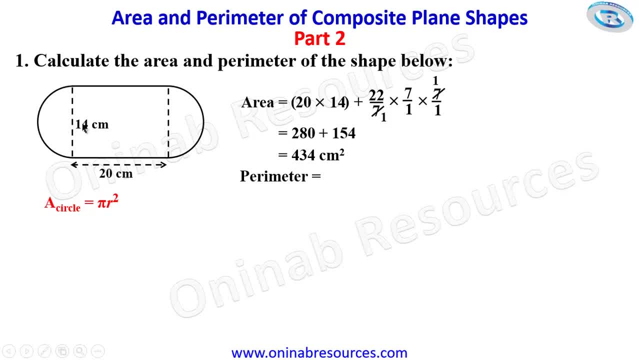 perimeter of the shape. To find the perimeter is to find the distance round the rectangle. We then go ahead and find the perimeter of the shape. To find the perimeter of the shape is to find the distance round the shape. It is not that you are going to find the 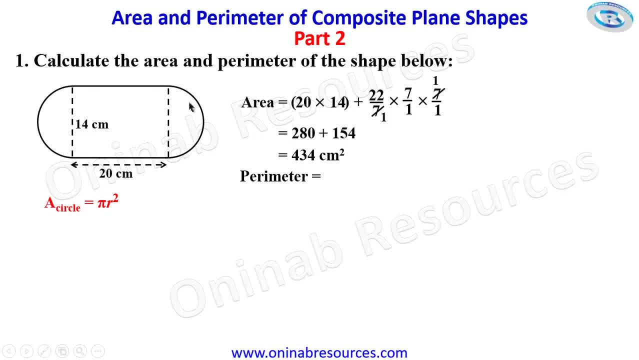 perimeter of the rectangle, find the circumference of the two semicircles and add them. No, We start from one point, then move round and add the sides and the semicircles. So starting from here now, this is 20 centimeters. So we have 20 plus the semicircle We are going to find the length of. 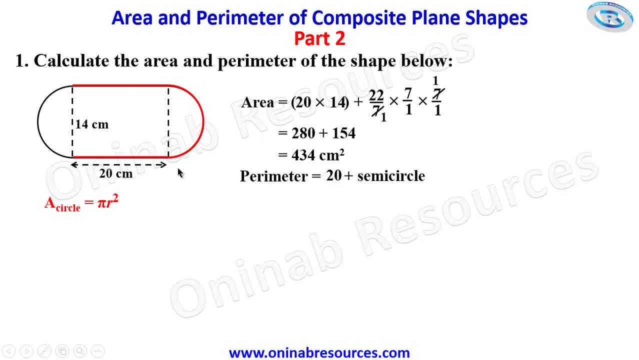 this semicircle then plus the length of this semicircle. We are going to find the length of this semicircle then plus this side again, which is 20 plus the other semicircle to give us the distance round the shape. So we add this 20 and this 20 to give us a 40. This semicircle and this semicircle. 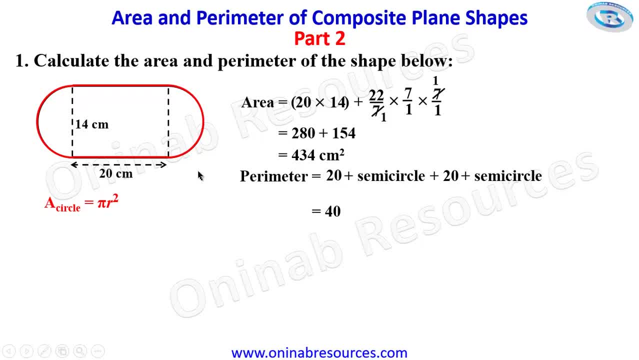 when added together, will give us a complete circle. We then find the circumference of the circle, So we are going to add the circumference of the circle. So we are going to add the circumference of the circle, which is pi d, and our pi still remains 22 over 7.. Our diameter here is: 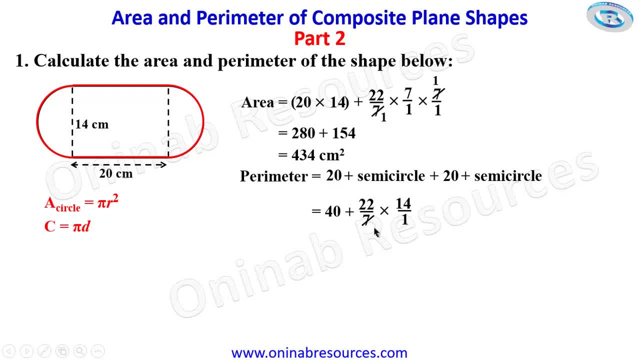 14.. So multiply by 14 over 1.. 7 goes into 7 gives 1.. 7 goes into 14 gives 2.. We then have 40 plus 44.. 22 times 2 gives 44.. 40 plus 44 gives 84 centimeters. 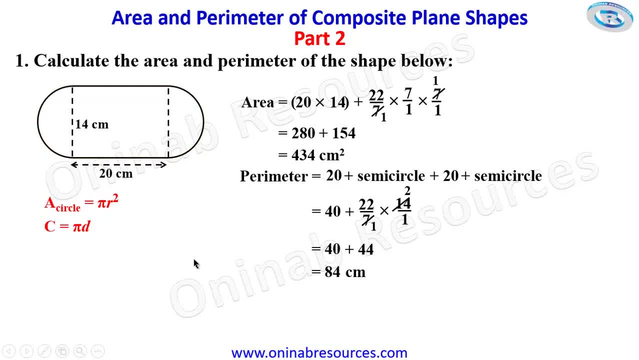 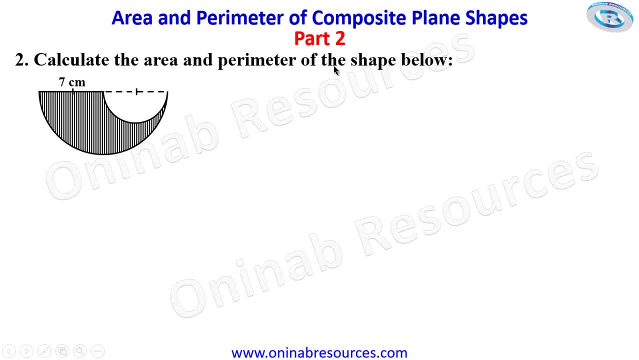 Host the perimeter of the circle which represents the perimeter of the shape. That's all for problem 1.. For problem 2, calculate the area and perimeter of the shape below. This shape is a combination of two semi-circles, Three larger than the other and a radius of 7. centimeters. A radius of 7 things is the Cot renovations together or different divisions of the triangle into a 3d pyramid. The radius of that larger semicircle is the diameter of the circle- 7 cm. and the radius of that larger semicircle is the diameter of the circle. I think there is one answer that you need to answer. neither here nor Bangor or theWhoa are both recognizing that theirbereich is 10 sunlight, then also a bit too high. So here is a formula: ط�. Just so I know. 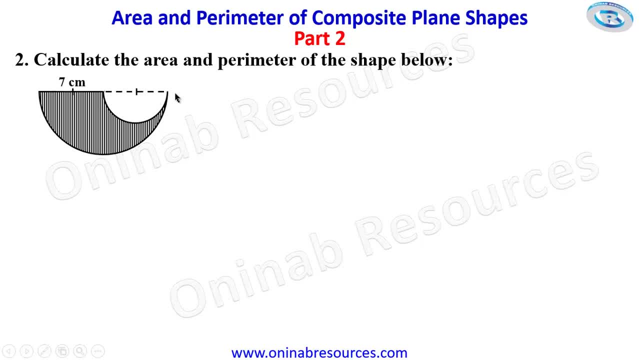 4.. In addition, I'm describing a three-dimensional curve. Both are not divided by 0, and then I cannot be determined a smaller semicircle. so to calculate the area, this is a case of subtraction. we find the area of the entire semicircle, then find the area of the small semicircle. we find the difference, so that we are: 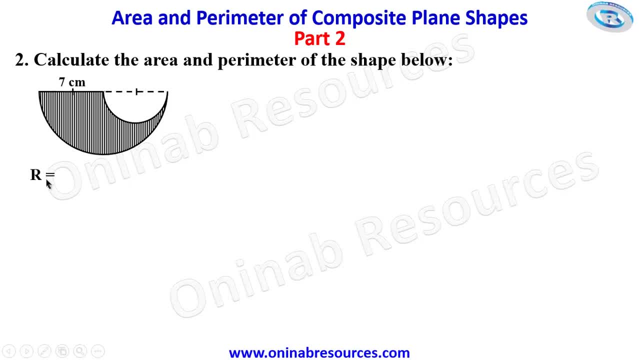 going to have the radius of the large semicircle, representing capital r, to be 7 centimeters and since the diameter of the small semicircle is 7, the radius will be 3.5. 7 divided by 2, this 3.5. 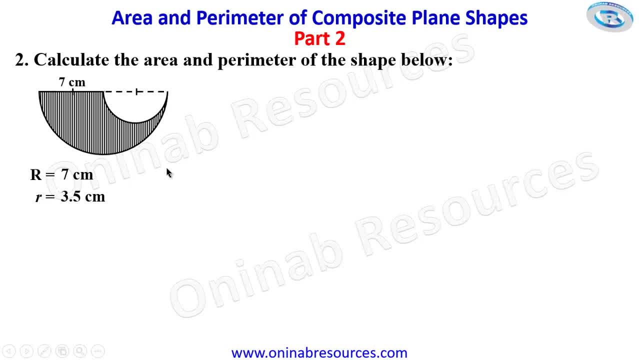 can also be written as three and a half or seven over two, so that the area of the shape now is going to be area of any semicircle, is half pi r squared. since pi r squared is the area of the small semicircle, and since the diameter of the small semicircle is 7, the radius will be 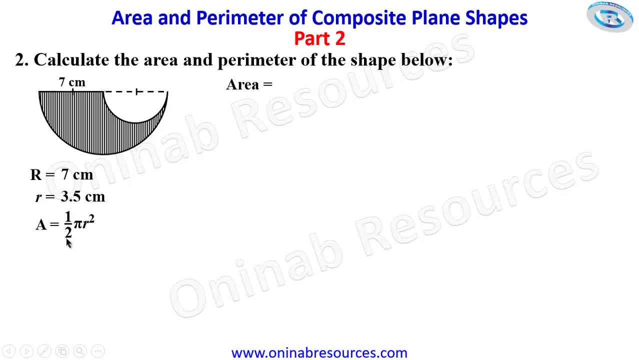 a circle. so since it is a semicircle, we multiply by half, so that we now have our area of the large semicircle as half pi, capital r squared minus half pi r squared small r. substituting into this formula, we have: 1 over 2 times 22 over 7 times 7 over 1 times 7 over 1, since the capital r is 7, then minus. 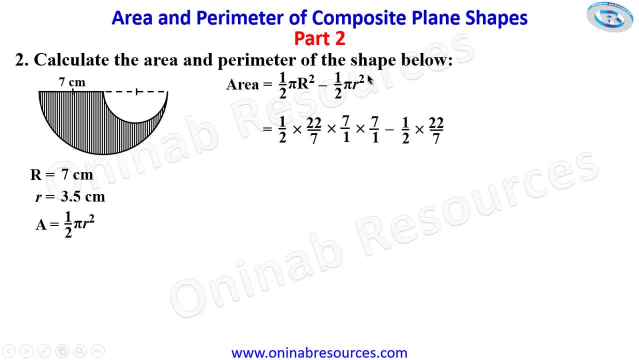 1 over 2 times 22 over 7. small r times 7 over 2 times 7 over 2. we informed you earlier that the radius of the small semicircle is 7 divided by 2.. so, simplifying here, 7 goes into 7: 1. 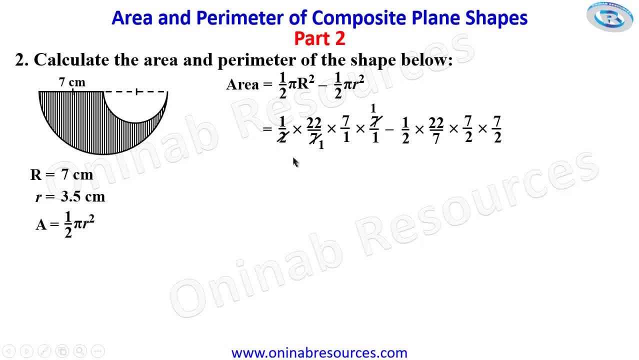 7 goes into 7, gives 1, 2 goes into 2. 1, 2 goes into 22, gives 11.. so 11 times 7 is 77 minus 7 goes into 7. 1, 7 goes into this. 7 gives 1, 2 goes into 2. 1, 2 goes into. 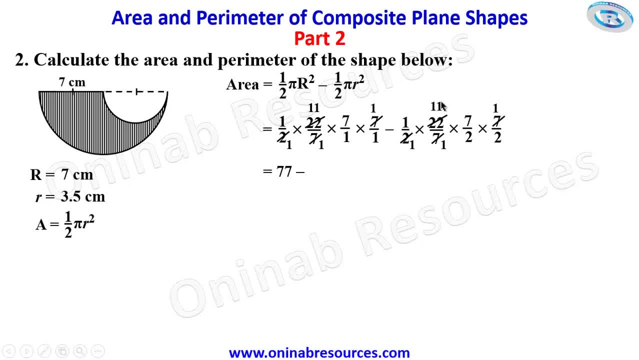 22 gives 11.. we are then left with 11 times 7. that's going to give us 77 over 4.. we then simplify. to simplify this, we find the lcfd to be 4.. uh, here is supposed to be original 77 over 1.. so we now have 4 times 77 to give us. 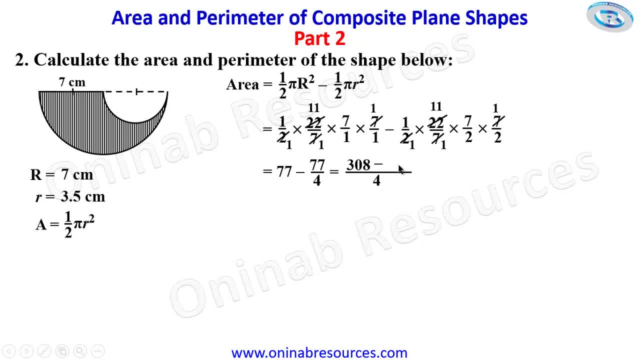 308 minus 77.. since four divided by 4 gives 1 times 77 gives 77.. 308 minus 77 gives 231. over 4, 4 goes into 23, five times remainder 3 in 31 is 7 times remainder 3, so that's going to give us 57 old. 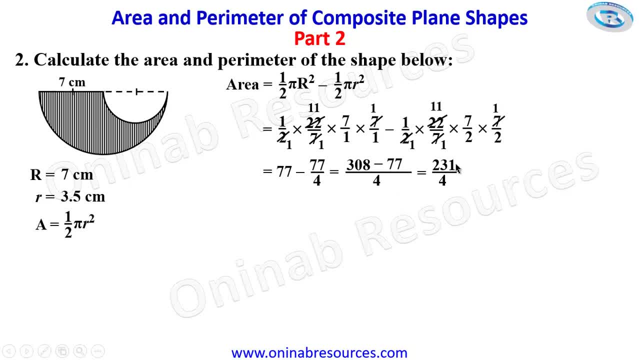 number 3 over 4, and that 3 over 4 can be written as decimal to be 0.75. so that's 231 divided by 4 gives 57.75 square centimeters, representing the area of this shape. we then go ahead to calculate the perimeter. we still 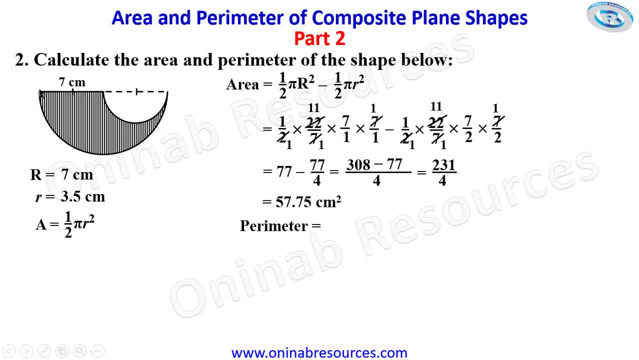 remember that the perimeter of composite shape of this nature is a distance round the shape. it's the calculation of the sum of the distance round the shape. so here is going to give us a 7, as from here to this place is 7 centimeters plus. 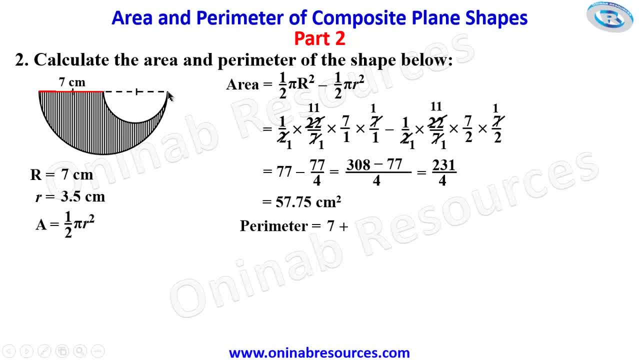 the next is the circumference of this shape, of this semicircle, and circumference of any semicircle is half pi d, so we have to get this. that's going to give us half pi d, small d, then. from here now to the starting point, that is going to be plus half pi d, capital letter d and that. 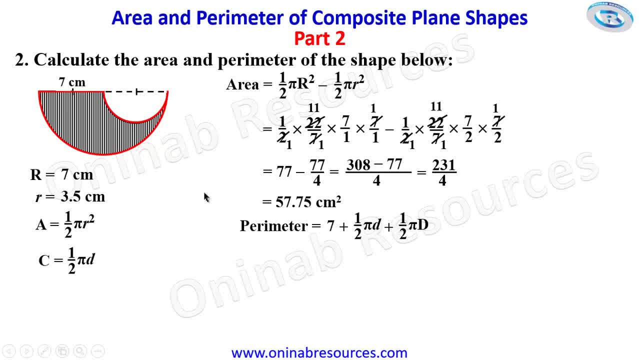 capital letter d is 14 centimeters, so substituting we have 7 plus 1 over 2 times 22 over 7 and our D, we said, is 7 from here to this place is 7 centimeters. then plus half times 22 over 7 times 14 over 1, 7 plus 7. so 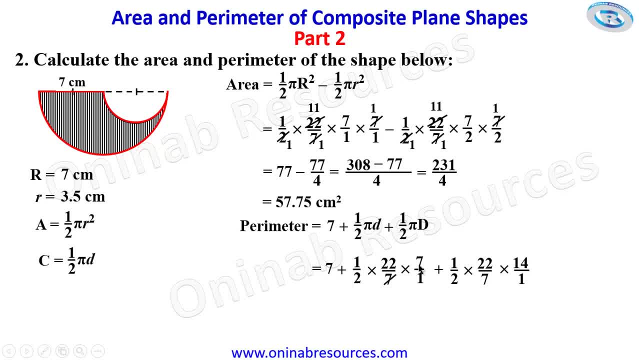 simplifying this, I have a this: 7 goes with this 7. 2 here. 1 goes in to 22 gives 11 here. 7 here: 1. 7 here gives 2.. 2 goes here: 1.. 2 goes here 1.. We are left with 11 here, so we have 7 plus 11. 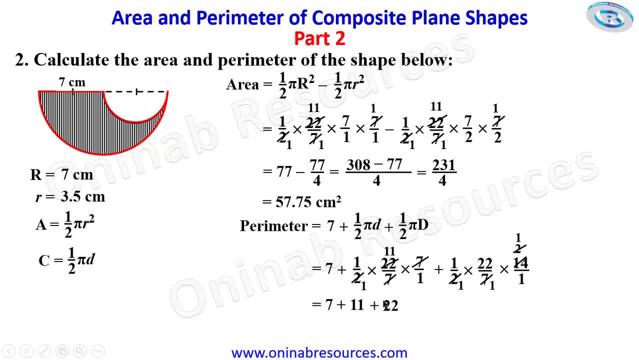 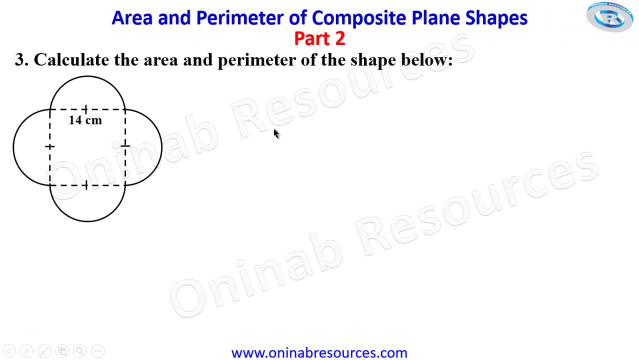 and we are left with 22 here plus 22. This is 33 plus 7, giving 40 centimeters as the perimeter of the shape. So that's all for problem 2.. We then go to problem 3.. For problem 3 we have: 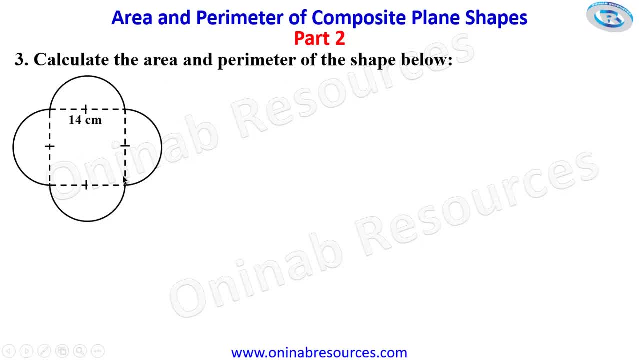 another composite shape comprising of a square and four semicircles and the sides of the square is the diameter of the semicircle To calculate the area. now we are going to calculate the area of the square And then the area of the four semicircles. we add them together, since the four semicircles 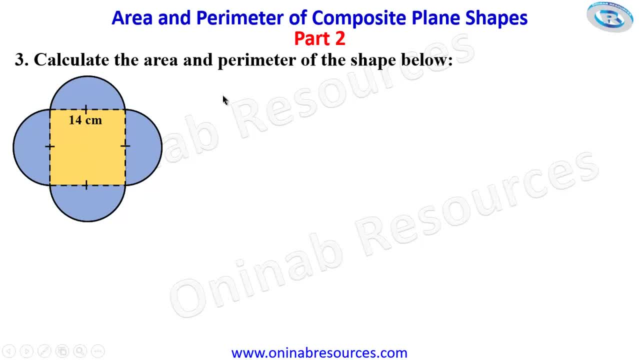 are joined with the square. So we start with the area to be area of the square plus area of the four semicircles. Area of the square is L squared and our L is 14, so we have it as 14 times 14 plus. 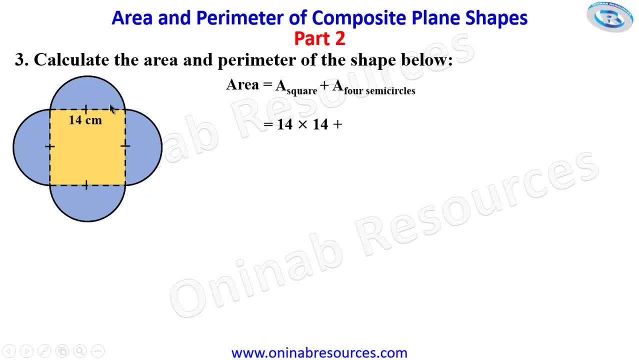 here we have two semicircles forming one, Two semicircles forming one, so in total we have two circles. So we now find the area of one circle and multiply by two, The area of a circle is pi L squared, so we have it as: 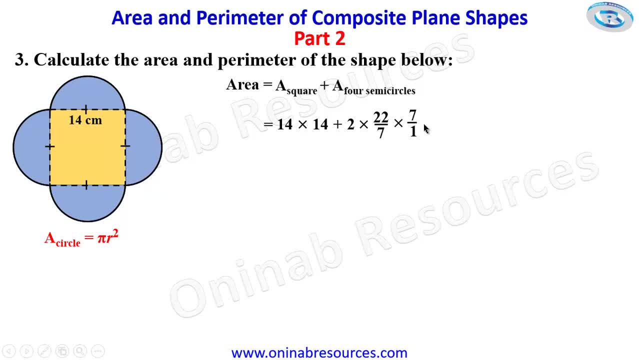 2 times 22 over 7 times 7 over 1 times 7 over 1. so seven goes into seven, one Seven goes into seven, creating 1, and we are left with 2 times 22 times 7 here, and for this we have 14 times 14, giving us 196. 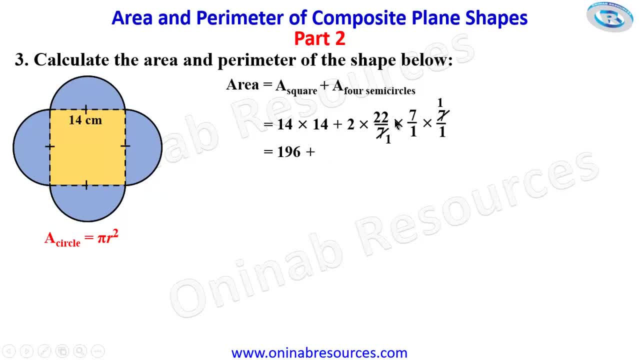 plus 2 times 22 gives 44. 44 times 7 gives 308. adding them together, we have 504 square centimeters representing the area of the shape, so that we now go ahead to calculate the perimeter. for the perimeter, we are going to find distance around the shape again. 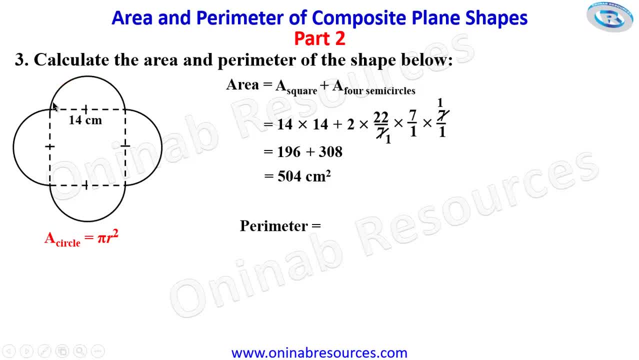 and starting from this point. so we have the first semicircle, then this, the third semicircle and the fourth one which is going to form circumference of two semicircles. so we know the formula for calculating the area of the shape and we are going to find the distance around the shape.